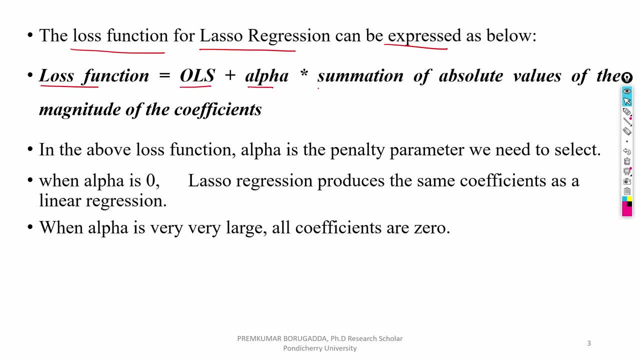 ordinary least square plus alpha, is multiplied with the sum of the absolute values of the magnitude of the coefficients, which means that so here the lasso, we can write like this: so, which means that the cost function, so 1 by n sigma i, is equal to 1 to n. 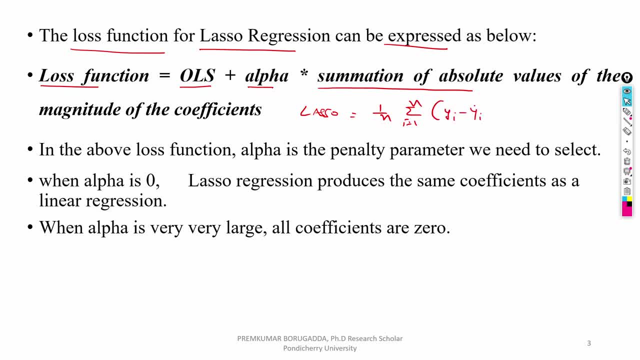 y i minus y hat whole square, plus lambda is multiplied with this m whole square. so here the loss function is equal to 1 by n sigma i is equal to 1 to n, which means thus: so this is the predicted variable. so here y i hat is nothing. but we can write like this: 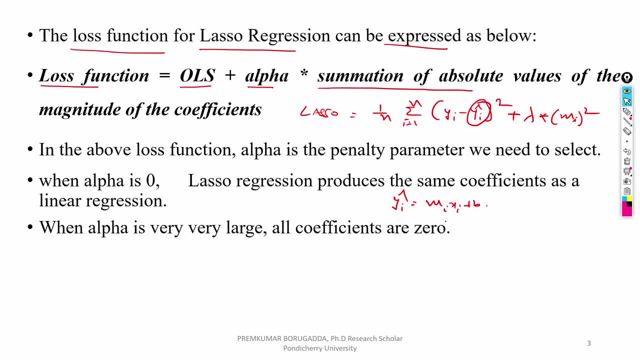 m i, x, i plus b, so, which means that so the loss function mean square error can be write like this: 1 by n sigma i is equal to 1 to n, y i minus y, i hat whole square. plus lambda here, sigma from i is equal to 1 to n m i, whole square. 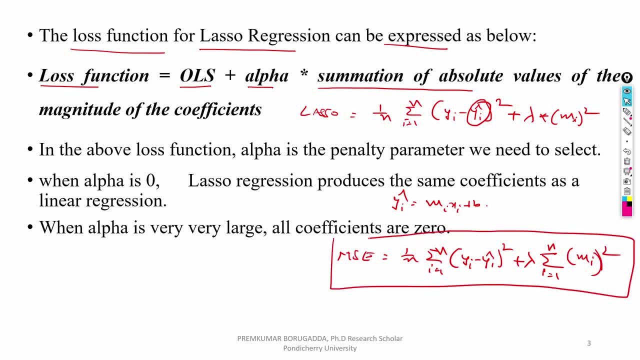 so this is the total loss function for this lasso regression. so in this loss functions this alpha is called the penalty parameter, penalty parameter. so this alpha value we have to choose manually. so whenever this alpha value is 0, so the lasso regression produces the the same coefficients as the linear regression. so what is the linear? 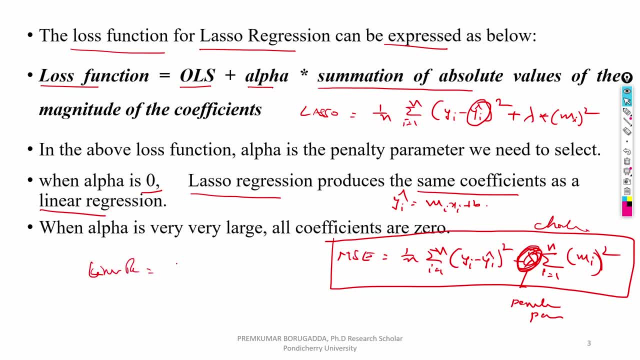 regression. so linear regression is nothing. but the 1 minus sigma is equal to 1, 2. here y i minus y i, at one square. so whenever the solve value 0, so this total, this value will be becomes 0. so which means whenever alpha is equal to zero, so the lasso regression, it becomes to the linear. 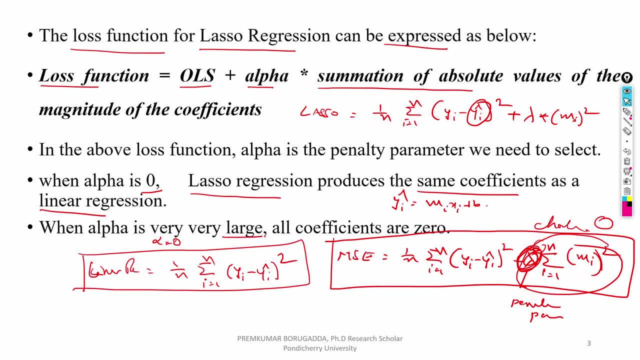 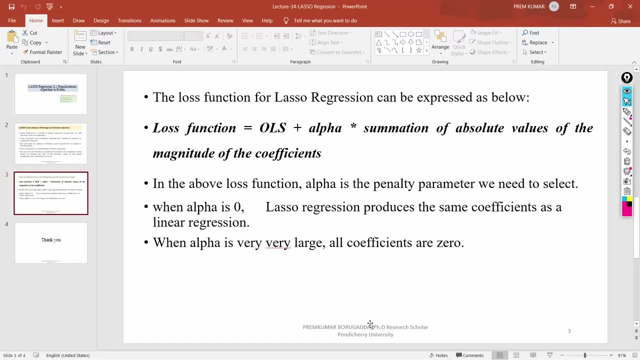 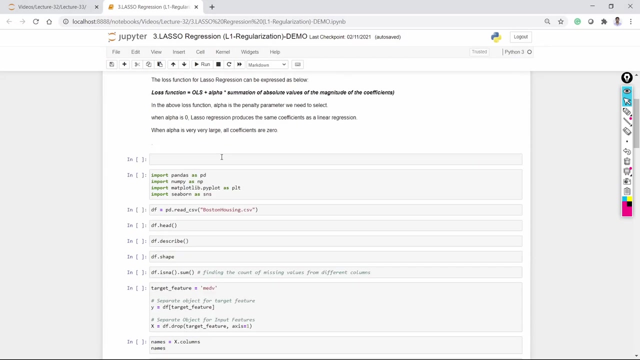 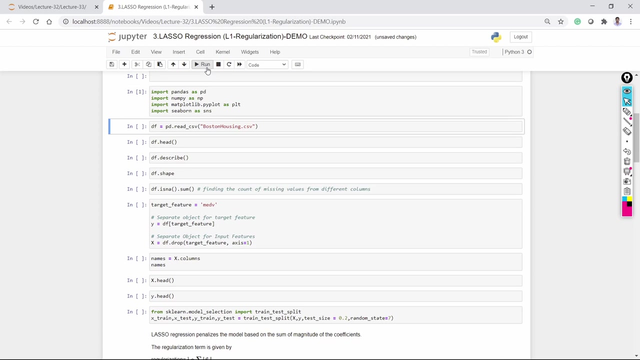 regression whenever this alpha value is very, very large. so at that time the all coefficients means m1, m2 and m3. so these are going to be zero. so this is the lasso regression. so now we are going to the practical section. so here i am importing the libraries, basic libraries, pandas, numpy, matplotlab z1. so i 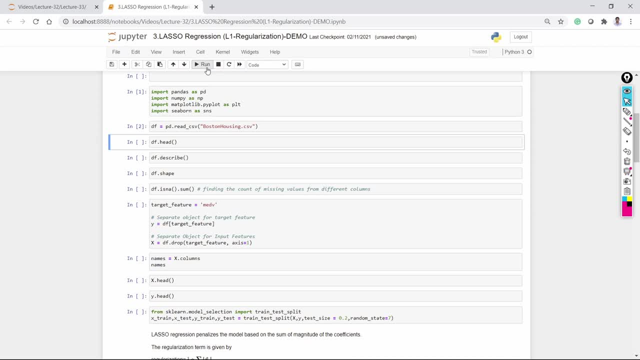 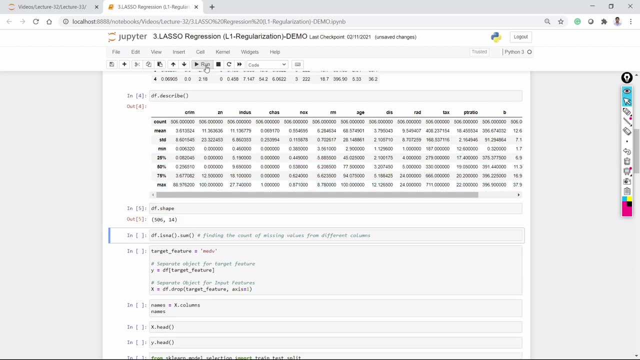 am taking the same data set which i was explaining in previous lecture, that is, the boston housing. so this is the head part and this is the statistical information of this data set. so, so, so data set shape is a final six observations and 14 columns. there is no null values so i can divide my 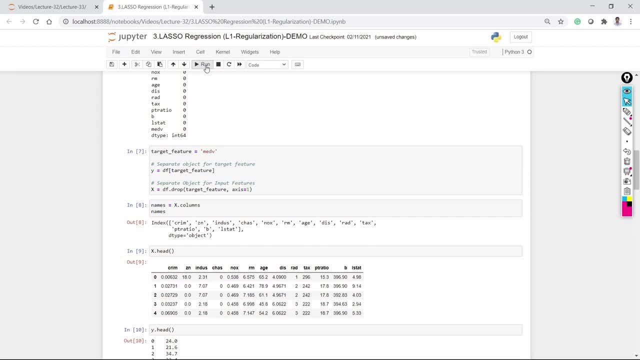 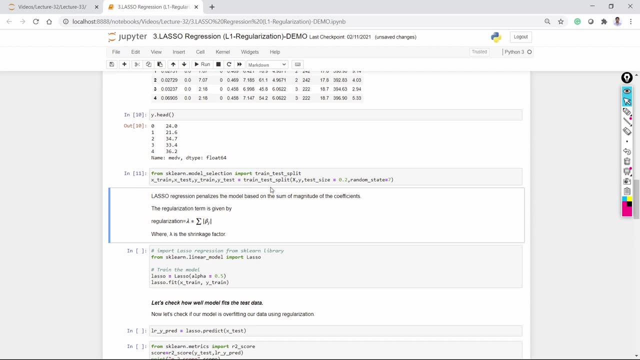 data set into independent variable and dependent variable. so then i divide my data set into train test fit, which means that my training data set is about 80 percentage and 20 percent is allocated for the testing data. so the lasso regression penalize the model. so, based on the sum of the 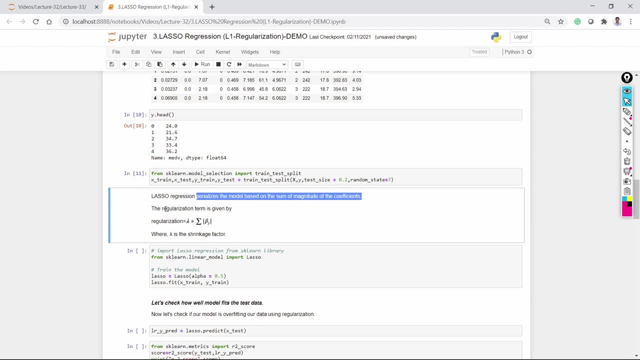 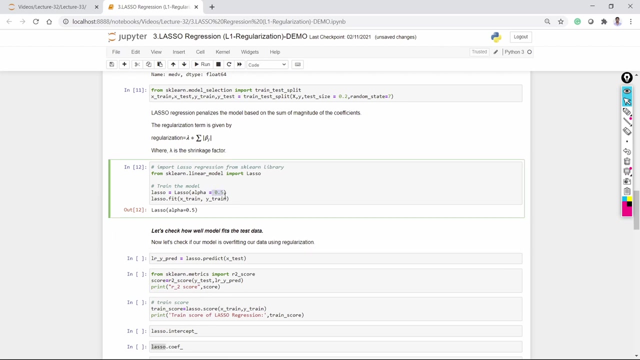 magnitude of the coefficients. so the regressionization term is given by. so what is mean by regularization? which means that so lambda is multiplied with the sum of the coefficients, of this sum of the magnitude of the coefficients. so here lambda is called the stinking factor. so here i am inputting the lasso and here i am taking the alpha value 0.5. 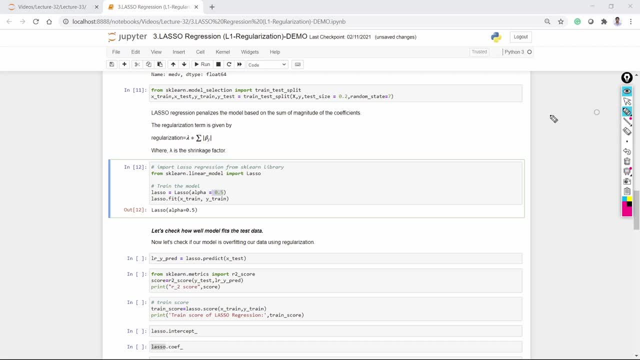 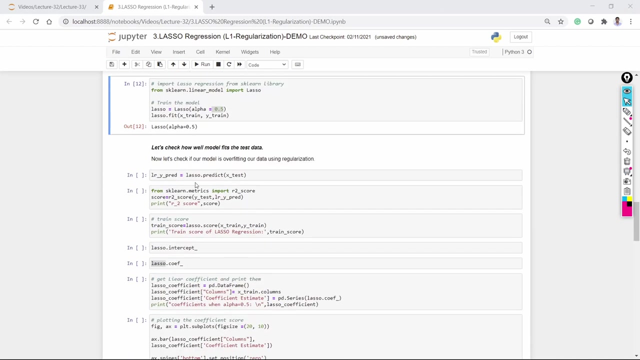 so you can take the alpha value. so you can take the alpha value from 0 to any positive integer. so here i'm taking the alpha value, 0.5. so now, now let's check the how our model is going to be fit on the test data. so i'm check the r2 score. 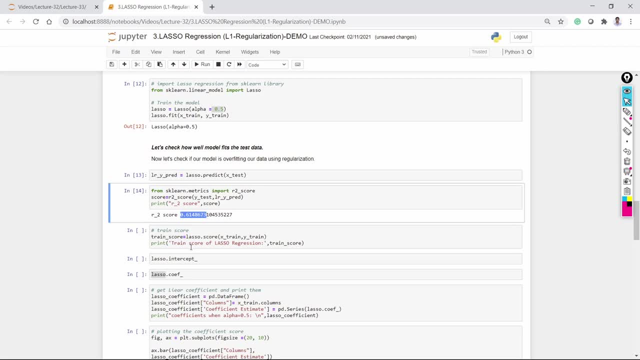 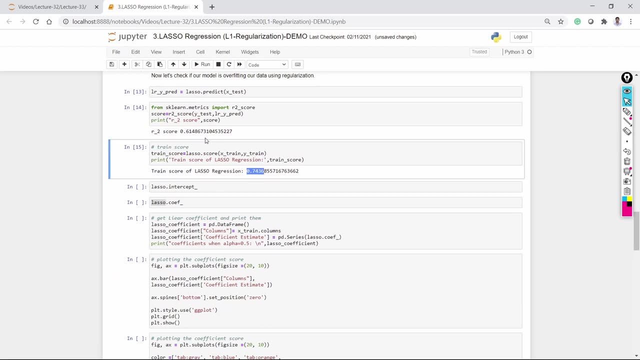 so i'm got. i got the 0.6148 when i check on the train score, so i got the train score 0.7436, which means whenever alpha value is 0.5. so i got this kind of results whenever you can check. 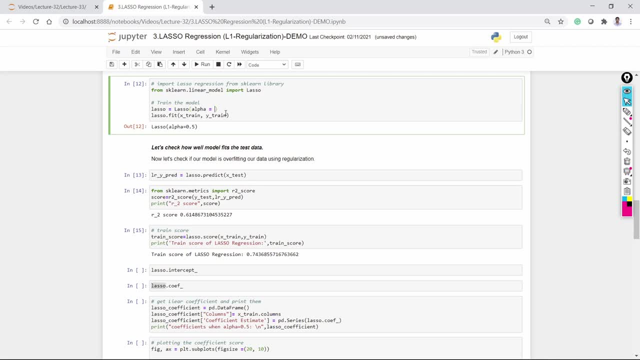 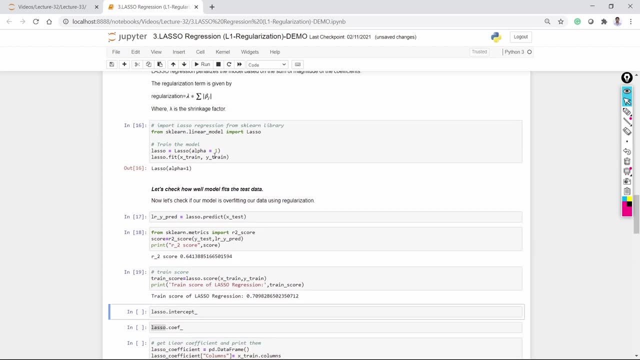 here you can choose the any value between 0 to any positive integer. suppose i'm taking alpha value 1, so again the results are going to change. so here i'm assigning the alpha value. so if place of 1 i'm taking the value 10, so again i'm executing, so results are going to change. 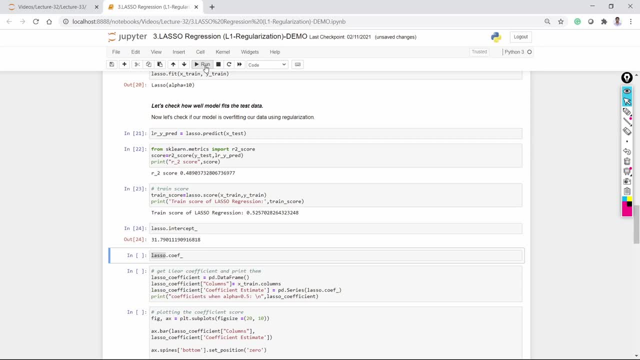 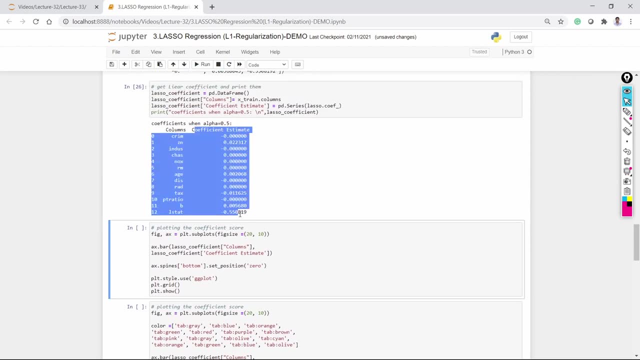 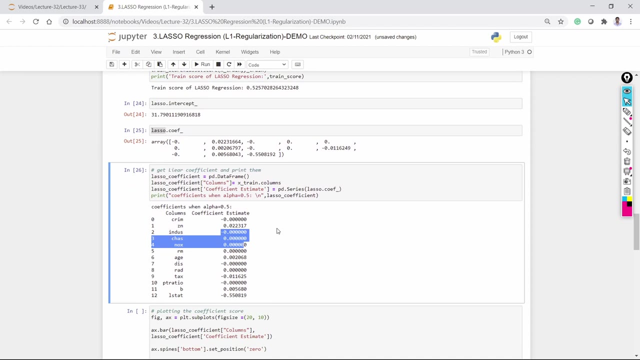 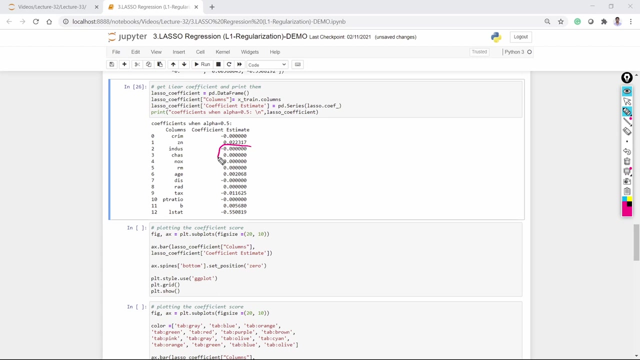 so if it is intercept, so this is the intercept value and this is the coefficients, and this is the coefficient values corresponding to these input values. whenever i mean changes my alpha value. so here, these some of the coefficients are going to 0, which means that all my value, so this is the coefficients- these coefficients are be 0, which 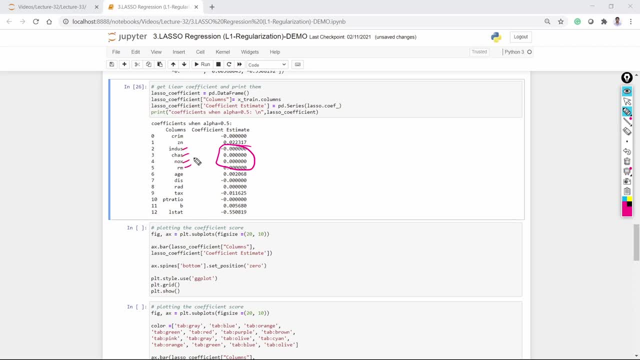 means these features, this feature, this feature and this features has to be eliminated. why? because these coefficients are be 0, so these two coefficients also will be 0 and this coefficient also be zero. so only what is the? this coefficient will be 0, so the what are the coefficients? or zero. 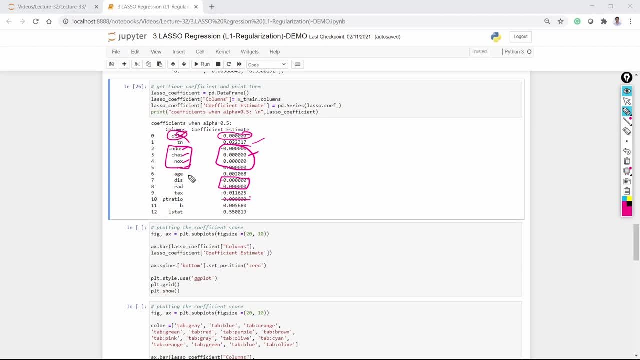 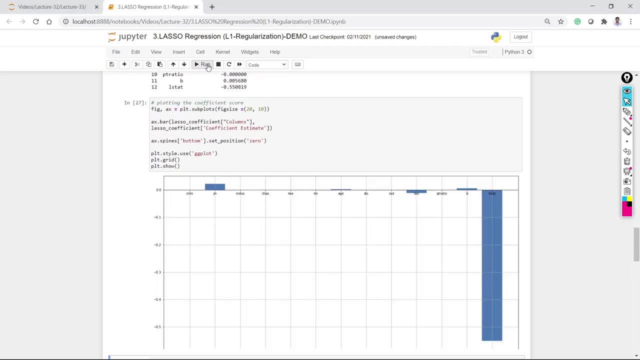 those corresponding features has to beischer eliminated from this data set, which means that we can select the best features for predicting the target variable. so that's why this lasso regression we can also call the feature selection technique. so here i plotting the. so whenever, see here. 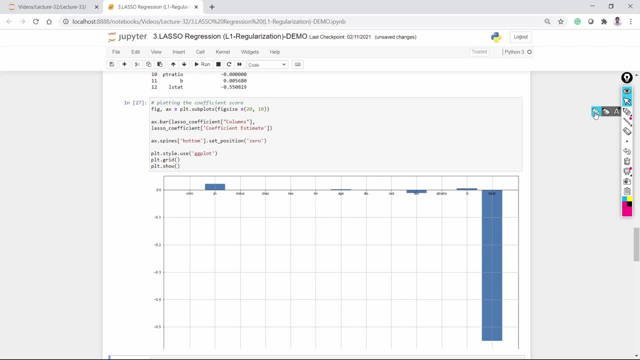 in this graph. so this is the zero. from here to here, from zero to downwards, it is a negative coefficient. values from zero to up, it is the positive coefficients. so here what is? the values are going to be zero. so these values are all zero values, which means the coefficients of 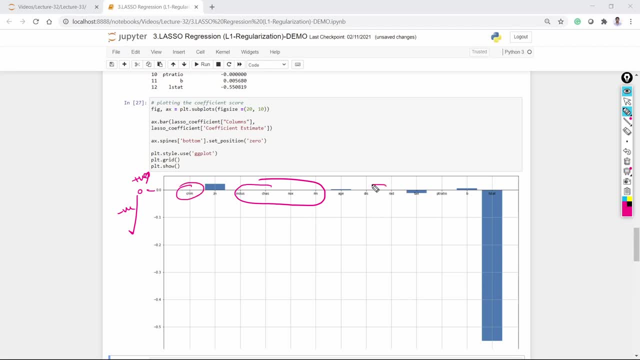 this features are 0, 0 and this is also be 0, so this, which means that this is the feature x1 and x3. this is x2, x3, x4, x5, x6, x7, x8, x9, 10, 11, 12, 13, so among 13 independent. 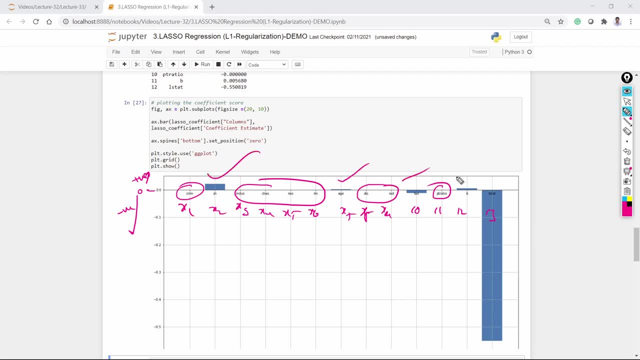 features: only this feature. 2, 3, 4, 5. this 5 features we are going to select for the predict in the target variable. so rest of the features are: coefficients are 0. that's why we have to remove this input features. so x1, x3, x4, x5, x6, x8, x9 and excellent. so these are the feature we are. 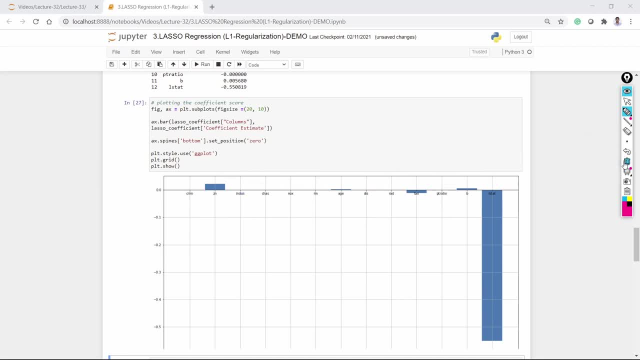 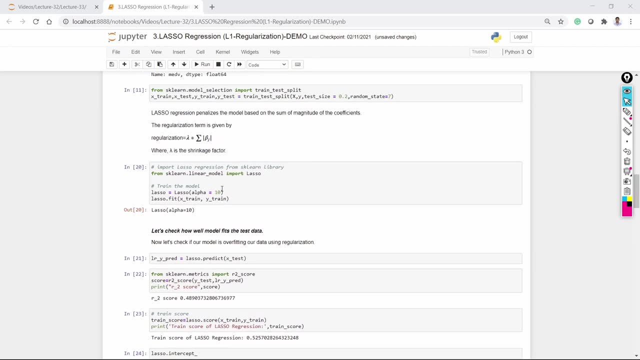 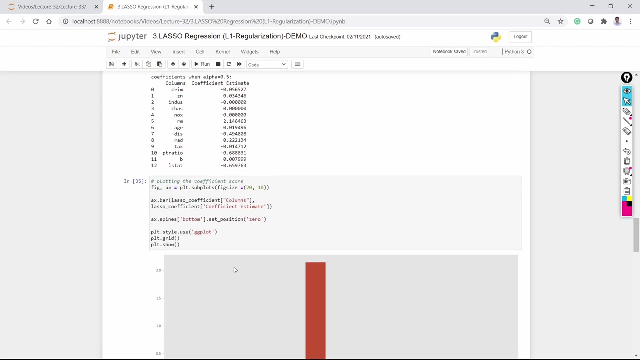 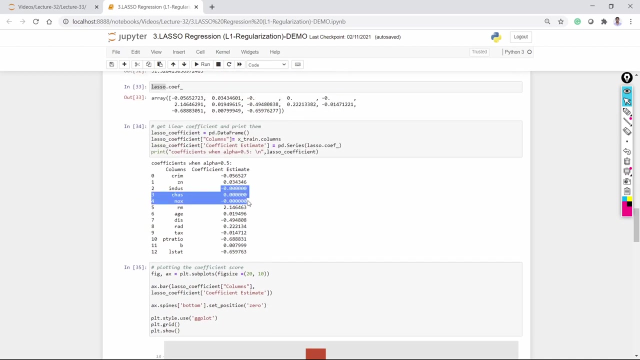 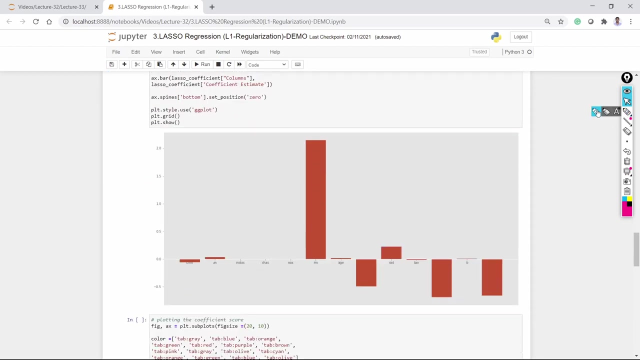 going to eliminate. so whenever, if you supposed to change this value, in place of 10, I am taking the value 1, so the values are going to change. see, coefficients are going to change. so here only some of the coefficients are be 0. only these three coefficients are 0, so others are. these values are existed, so which means that. so these 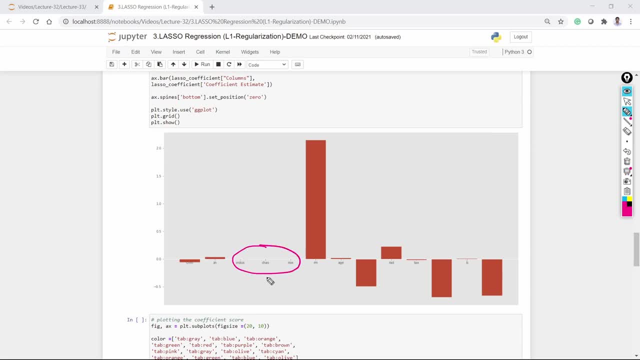 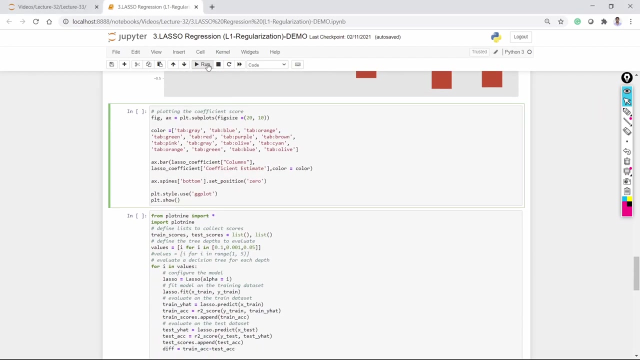 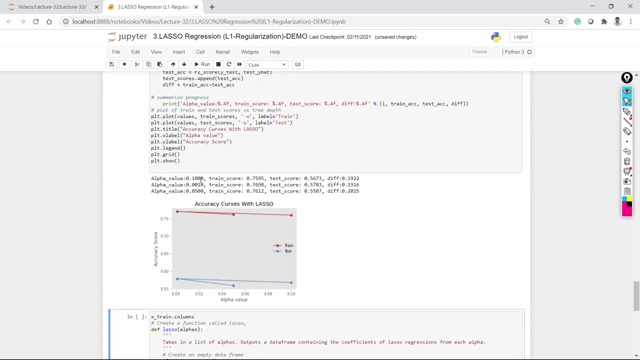 coefficients are only 0, which means the three coefficients are only 0. so rest of the coefficients we have to consider for predicting the target variable. so that's why in regression kind of algorithms, class of regression is very, very important for feature selection techniques. so here what I'm doing. so here I don't know which alpha value I supposed to. 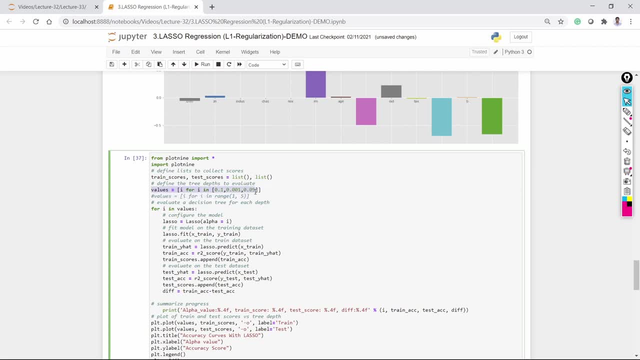 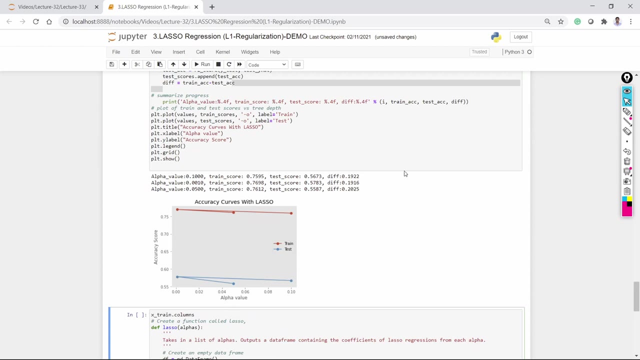 choose. so that's why I choosing this: some range of values. so I'm taking the alpha 0.1, 0.001, 0.05, 0.05, and I will plot this graph in this graph here. so in this graph, this is the X value. on x-axis, I am taking the alpha values and on y-axis, 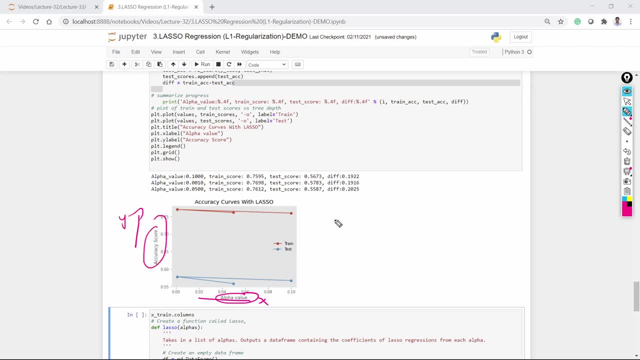 I am taking the accuracy scores. so accuracy scores are train score and test score. so here, this is the train score and this is the test score. so whenever: alpha value: 0.101, so this is the train score and this is the test score. and the difference between train score and test score is like this. so it 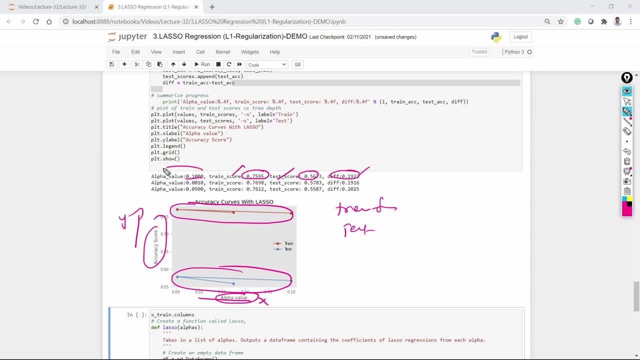 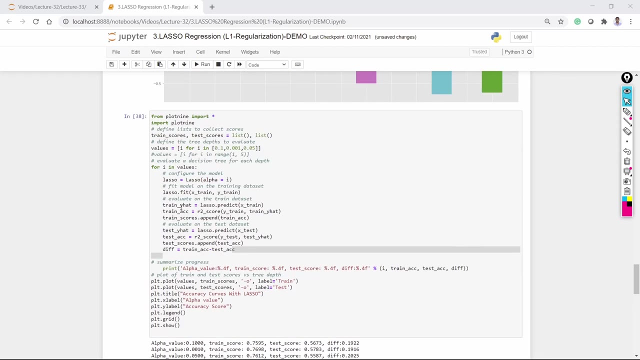 depends upon the train score, test score. it depends upon the totally alpha value. whenever alpha values, what kind of ranges you supposed to provide here? so according to that, you will get this train score and test score, suppose. let me check, I will give some other values. so here I'm passing. the alpha values range from 1 to 5, range from 1 to 15. so if you see alpha value, 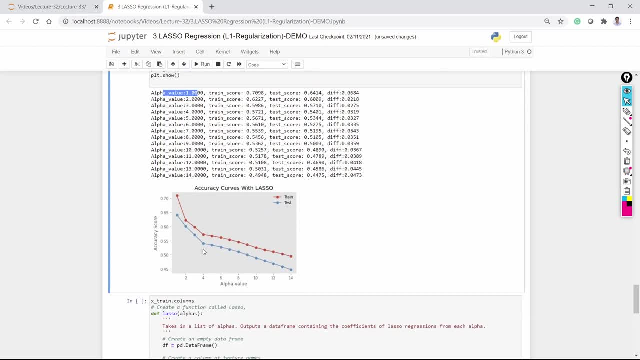 it 1. this is the result you got. so whenever alpha value is going to increase, so the train Score and test score are be decreasing. so here alpha value is going to increasing, so the train scoring will also be decreasing. so here alpha value is going to increasing, so the train score is also be decreasing. 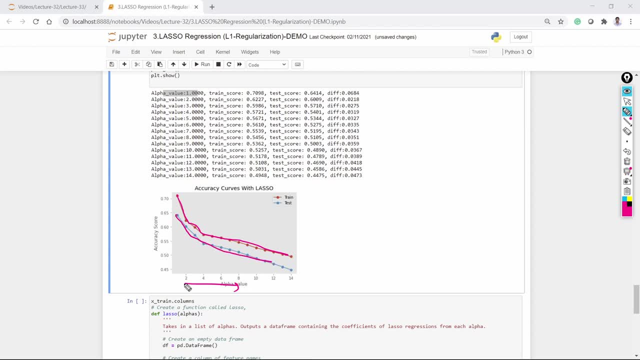 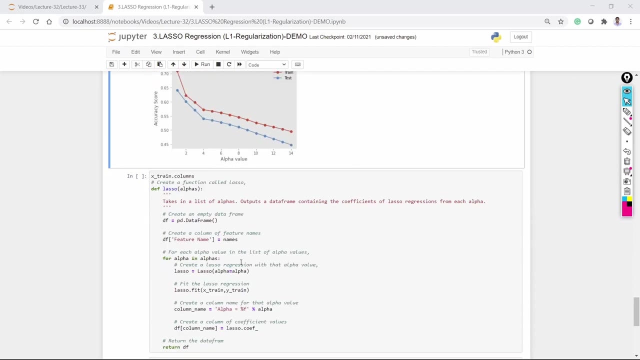 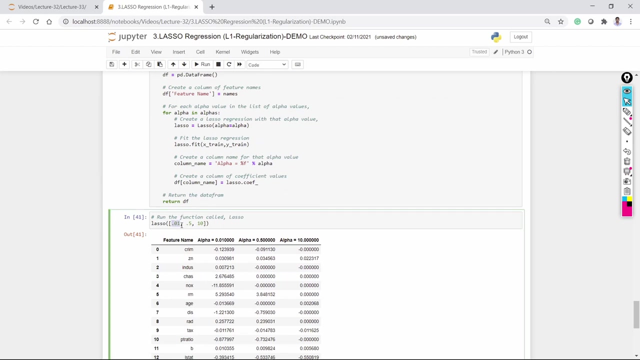 this is test score- also be decreasing. so, which means whenever alpha value is going to increasing, so this accuracy is trend score and just score- going to be decrease. if you see, if you pass this values like 0.1. so in this graph, in this diagram, in 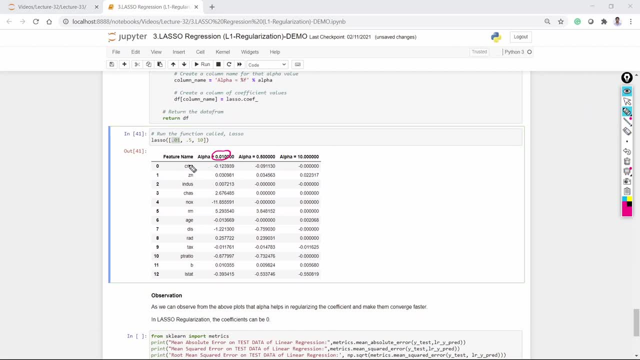 this output. so whenever alpha values 0.1. so this input x 1, x, 2, X 3 up to X 13, so this is the input value. like this: whenever alpha value 0.5. this is the m1 value. so pye, this is the m1 and this is m2 and this, sorry, so this is the m1, this. 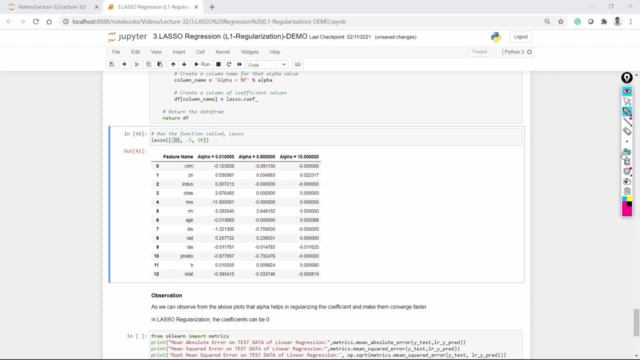 is m2 and 3 like that. so whenever, whenever alpha value is 0.10. so this is the x1, this is m1, this is x2, this is m2, whenever alpha value is 0.5. this is the result you got. so these are the coefficient. 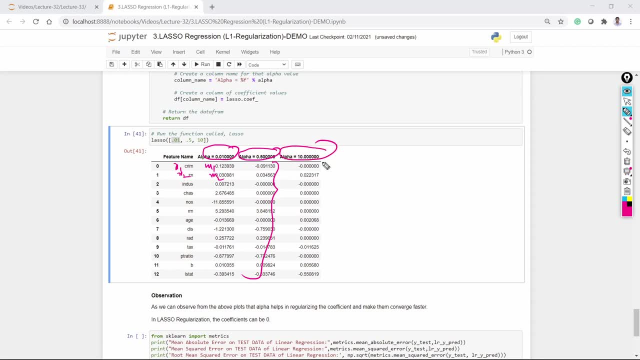 values. so whenever alpha is value going to increasing, see the results are going to change. so most of the coefficient are be 0. so this is the corner and value 0. so compare to alpha value 0.01. so the alpha value 10 is going to 0, which means that whenever alpha value 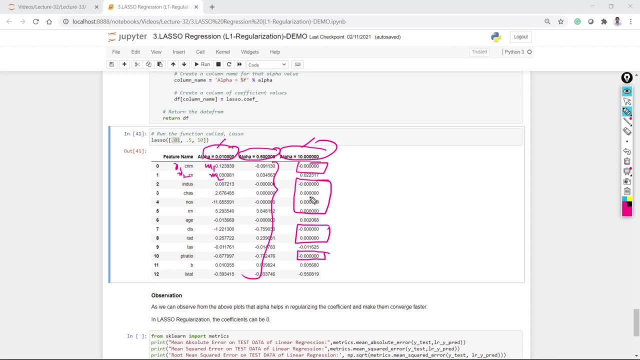 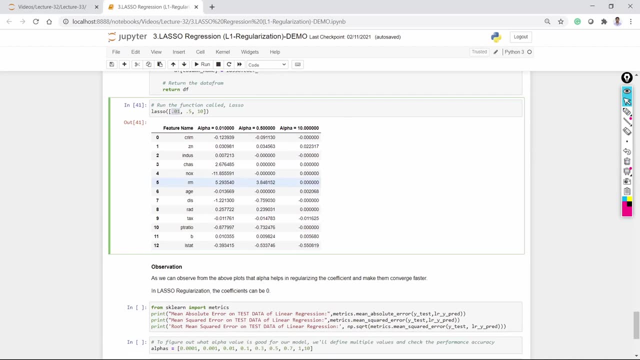 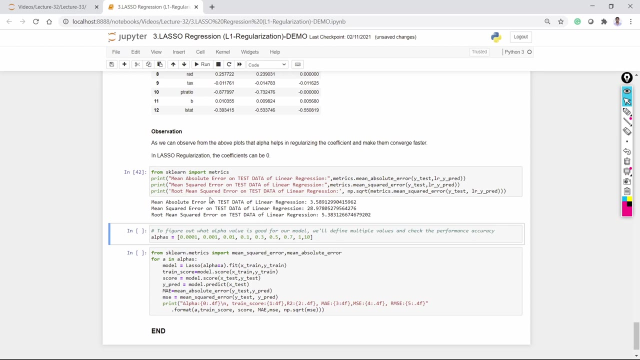 is going to increasing, so the coefficients are. the coefficients are going to be towards 0. it means he able to 0 ANY END. SO so this is the matrix. other matrix like mean absolute error, mean square error and root mean square error, suppose in this code- here i am taking the some values like alpha value. 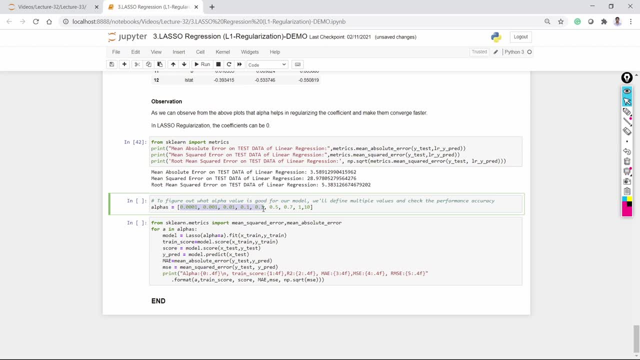 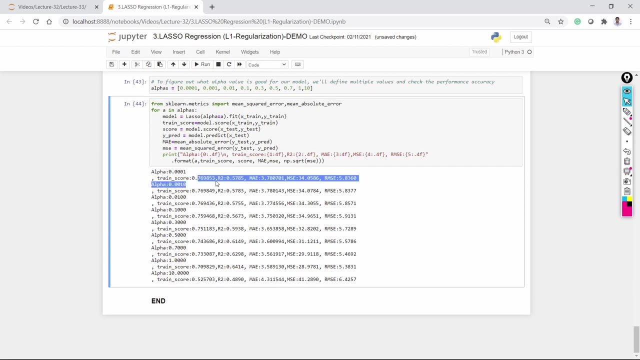 0.01, 0.001, 1, 3, 5, like that. so you can take alpha value, any value, from 0 to any positive integer. so i am taking some of the coefficient alpha values. so if i execute this code, so whenever alpha value zero, point 0, 1. so this is my time score and this is my r2 score. this. 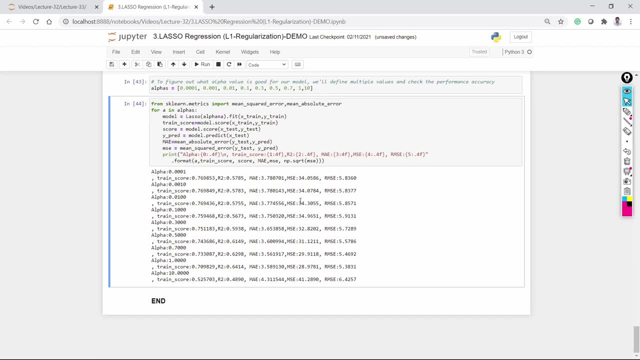 is mean absolute error, mean square error. root means square. so here you can clearly observe that whenever going to change the alpha values, the correspondingly the results are going to be changed. but you have to observe one thing here: alpha value is the hyper parameter value, so this is the 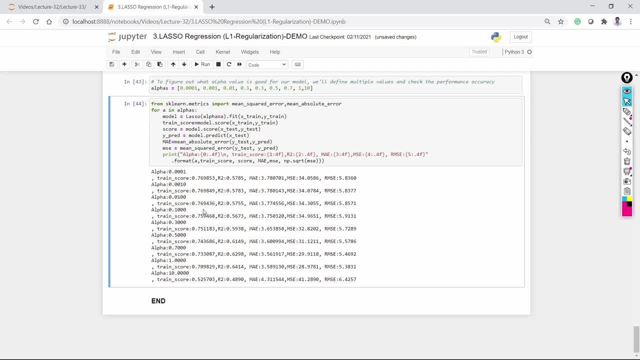 manually value here have to select this value. this value between 0 to any positive integer. so lasso can be used when we have more number of features. suppose in our data set more number of features are there, for example 100 columns, 200 columns, 500 columns, so at that time, so this lasso algorithm can. 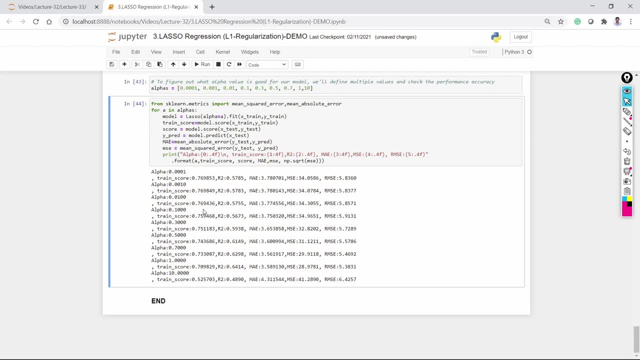 automatically do the feature selection. but what is the problem with this lasso when we have correlated features? when we have correlated features, so it retains only one feature. for example, there is a x1, x2, these are the two features, so these two features are being correlated. so m if two features. 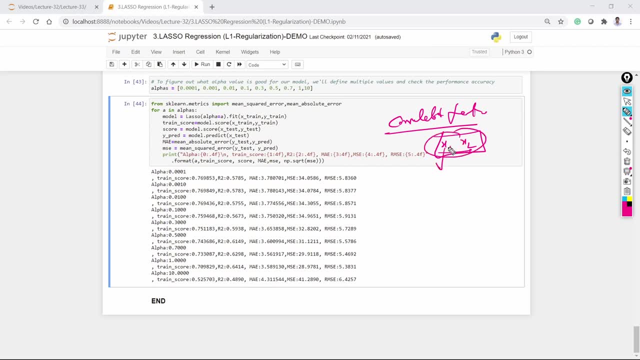 are be correlated. so here we have to choose any one of the feature, either x1 or x2. so if you choose x2, we have to drop the x 1. why? because what are the information is provided by the x1 feature. the same information also provided by the x2 feature. that's why we have to 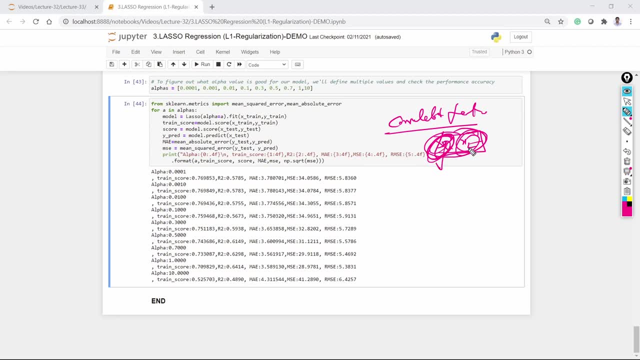 choose any one of the feature and drop the other feature. so if you drop the other feature, there is a drawback that there is. we have to log this, some kind of information. so we have to log this some kind of information. that's why, whenever we have correlated features, so only one variable, it has to be a set to. 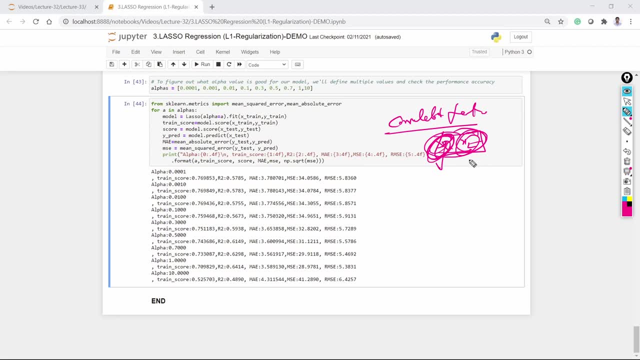 zero. another variable you have to be pick up so this will leads to the sum of the. so if you pick up this one variable and drop the other variable, so there is a loss of information and automatically you will get the less accuracy of your model if we have very few features of the data. so and the score is very poor. 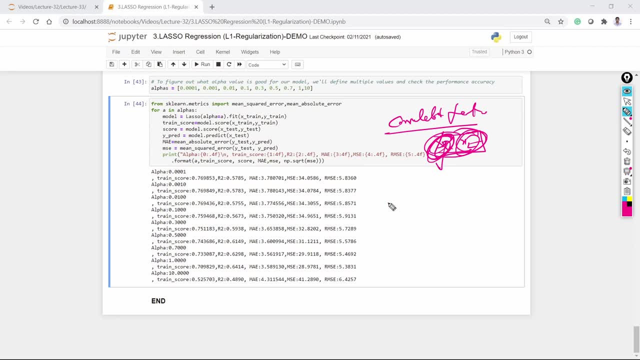 for the both training and testing score. if you have very, very, very, very few features, means number of features are very less. so at that time you will get the train score and test score very low. so at that time the model will be under fitting, under fitting, so whenever it is going to under fitting, 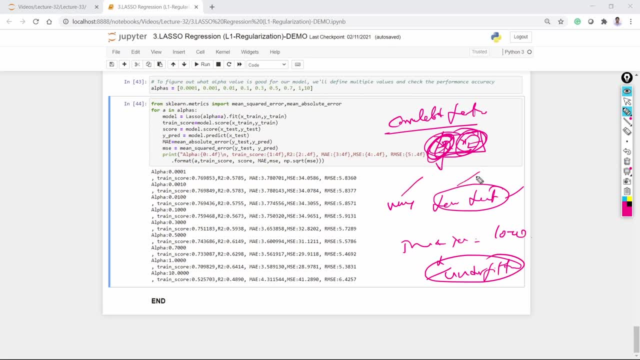 whenever we have the very, very few number of the features. at that time you will get the lesser training score and the lesser test score, which means that you are getting the very, very low training score. So imagine the model is a bit paid. it will get more features and then you will get. 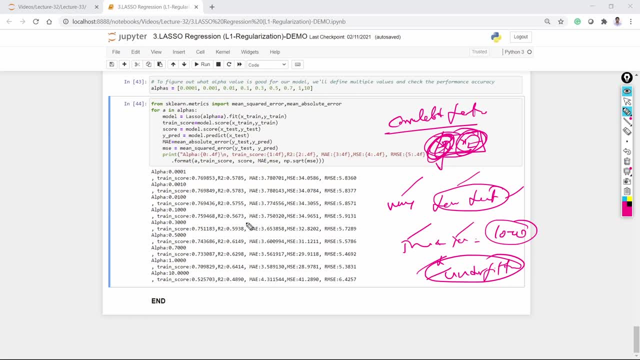 the lower scores and then you get again. they will have only one standard subt emerging. so at that time you can easily anticipate one individual item: that patient being netting. this is its only não, what is known as a Tieres. so this is the situation used to call overfitting. if you take very, very few data, underfitting may.